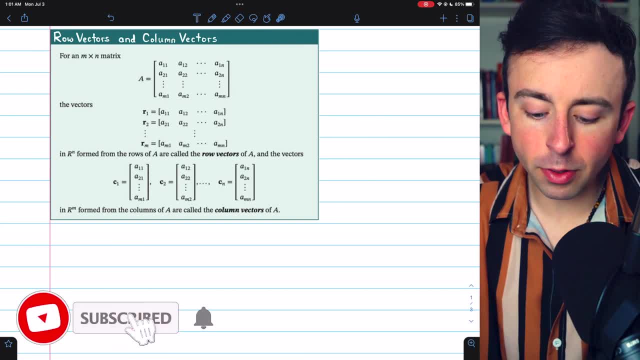 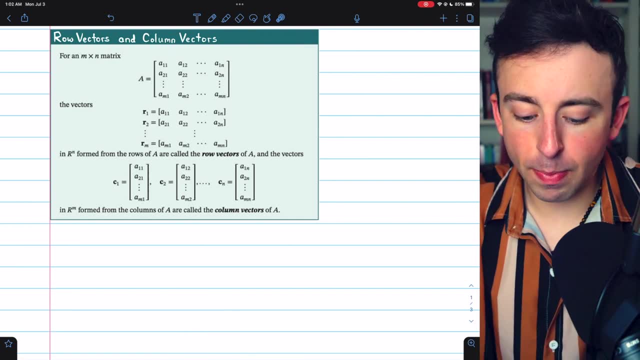 We can think of a matrix as being made up of row vectors or column vectors. Here's the definition of those terms from Howard Anton's linear algebra text. Just as you would expect, in an m by n matrix, the vectors in Rn formed by the rows of the matrix are called the row vectors. Remember. 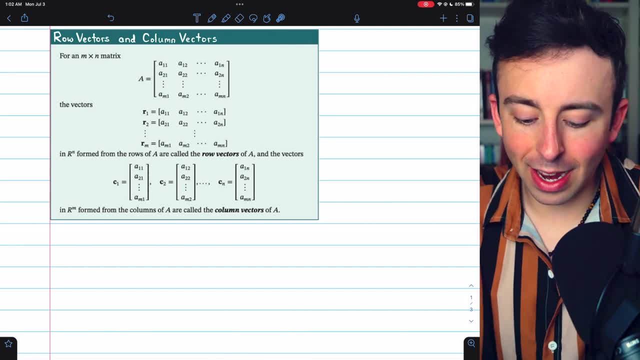 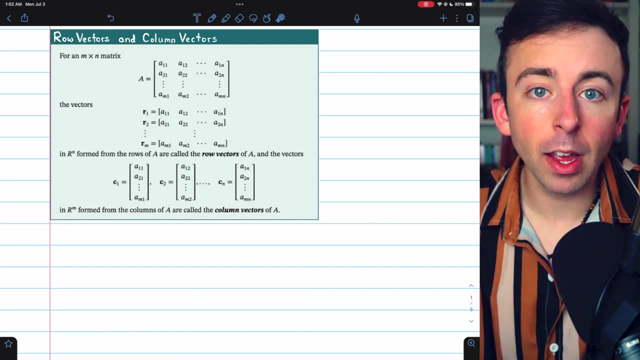 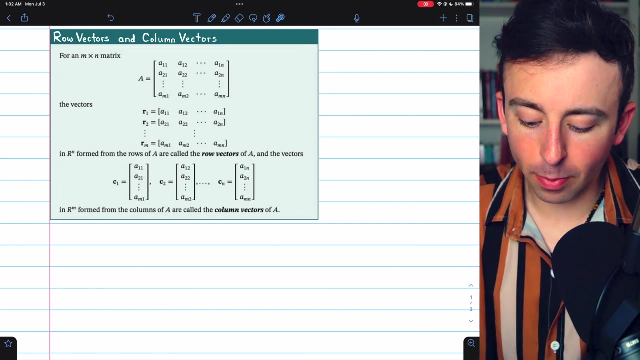 if the matrix has n columns, then each row will have n entries, which is why the row vectors are in Rn. On the other hand, each column would have m entries, the number of rows. so the columns of the matrix make up the column vectors and those are in Rm. The definition. 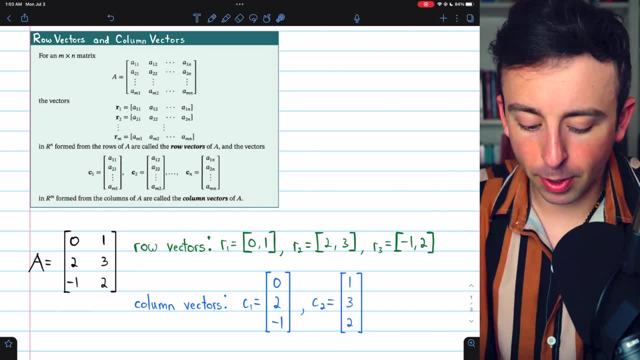 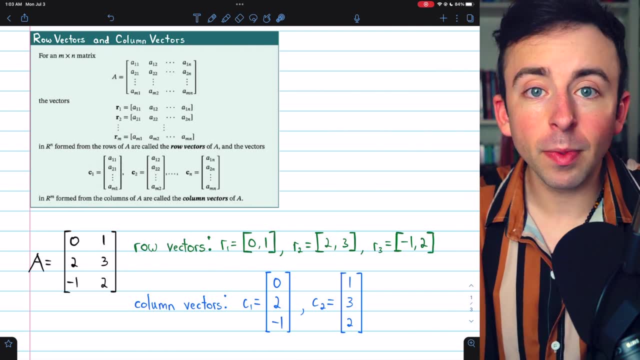 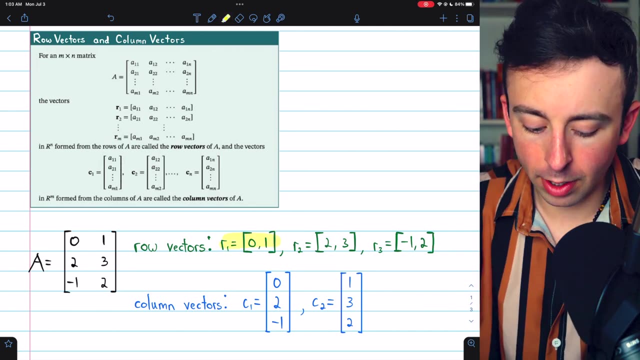 then, is exactly as you would expect. Here's a quick example. Here's a matrix A: It is 3 by 2, so each row consists of two entries and each column consists of three entries. Here are the row vectors of A: r1, this first row, r2, the vector for this second row, and r3, the 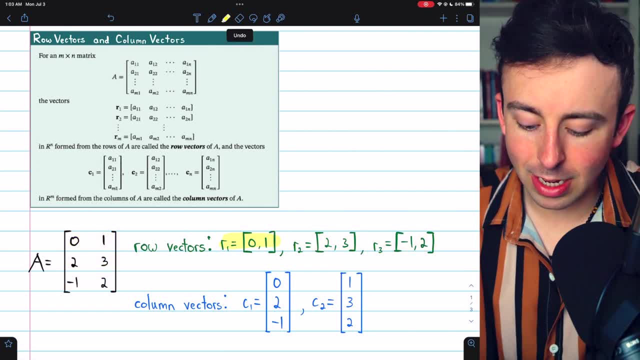 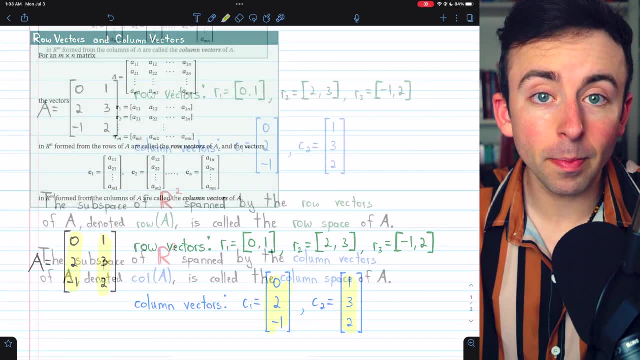 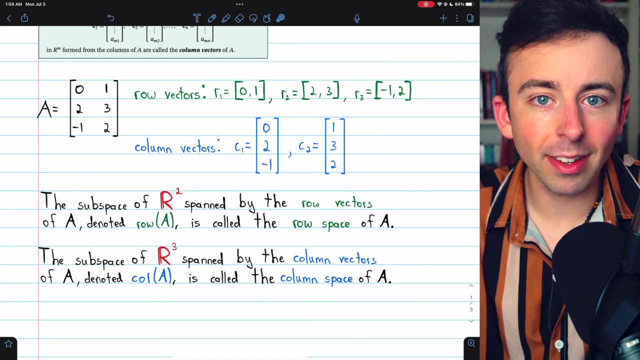 vector for the third row. Similarly, we could list out the column vectors. Here is c1, the first column, and c2, the vector for the second column. Perhaps the most important part of row vectors and column vectors are these things: the row space and the column space, which we'll talk. 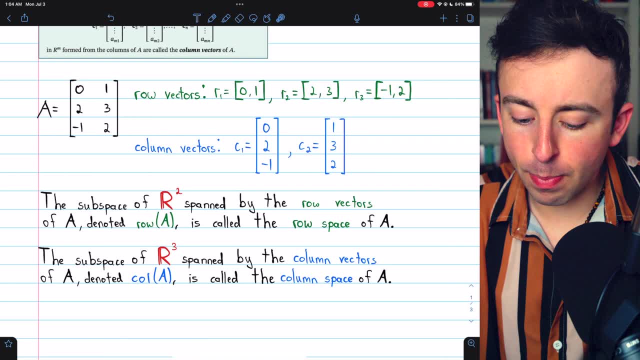 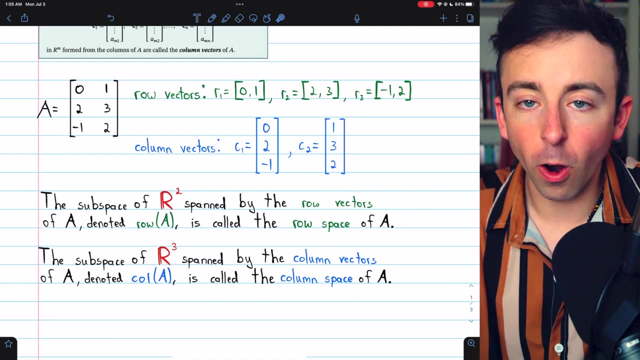 about next time. R2 spanned by the row vectors of this matrix A is denoted row of A and it's called the row space of A. Again, this is specific to this matrix A. That's why this is a subspace of R2,. 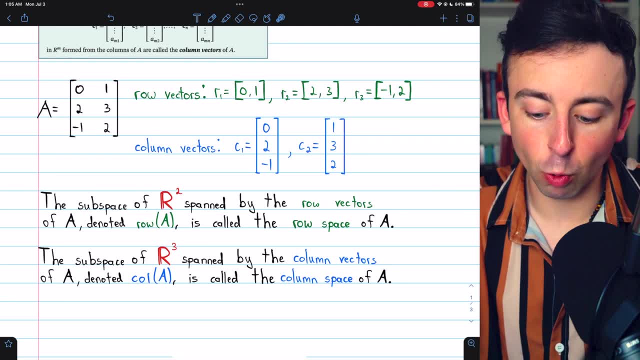 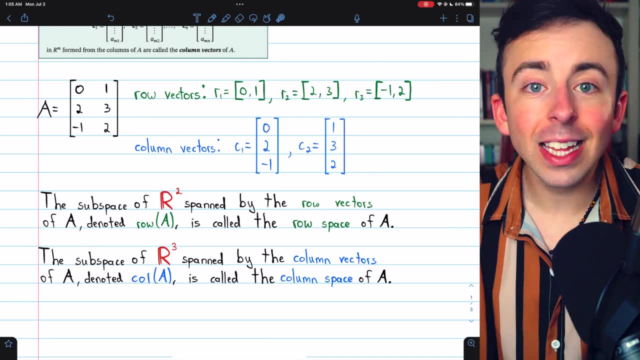 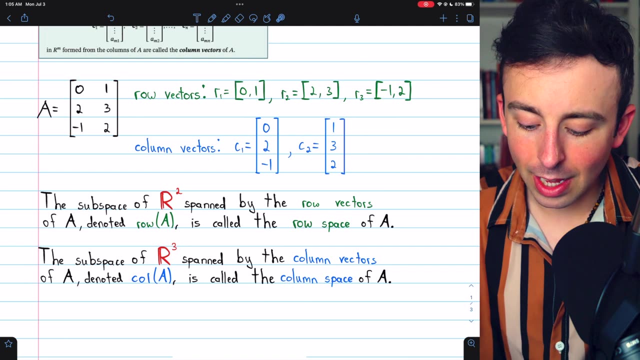 because A has two columns, so each row has two entries. And again the subspace of R2 spanned by these row vectors, that's what we call the row space of the matrix. Similarly, the subspace of R3 that's spanned by the column vectors of our matrix, A is denoted call of A and it's called